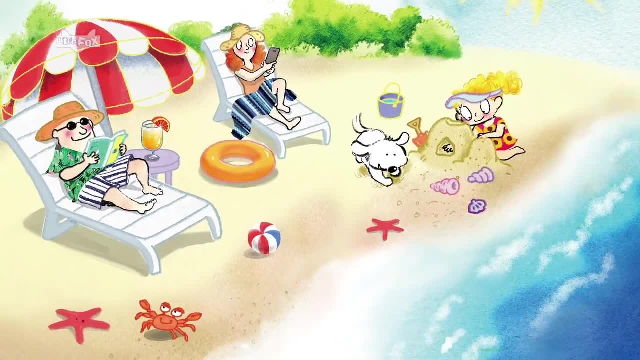 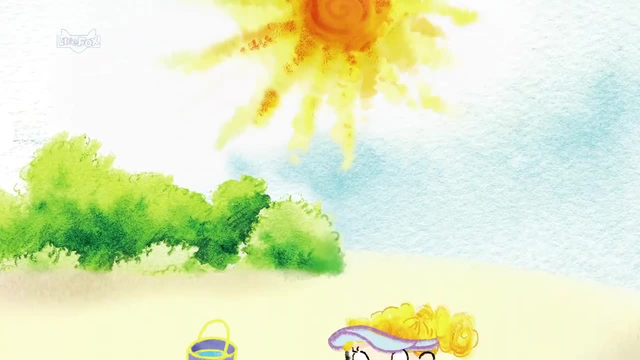 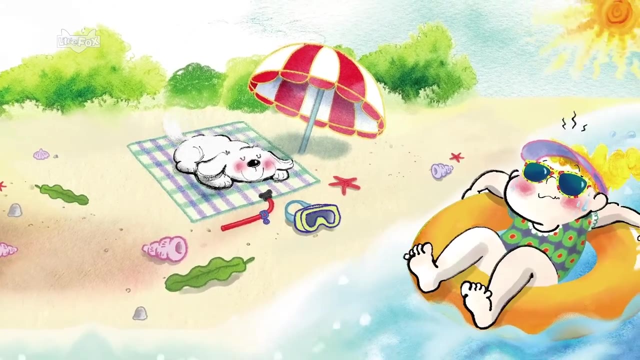 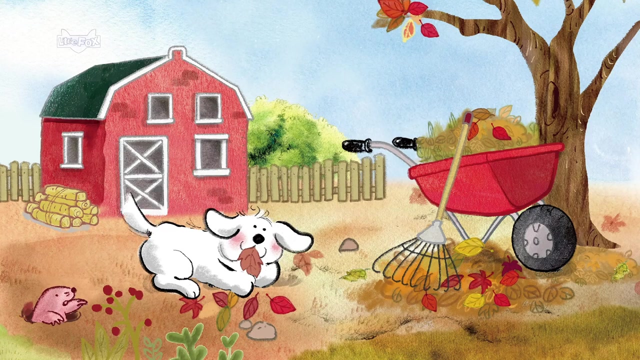 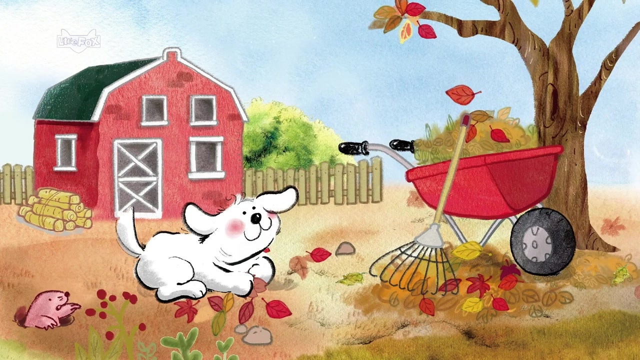 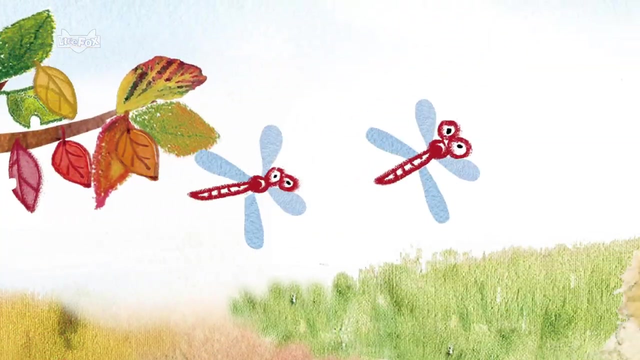 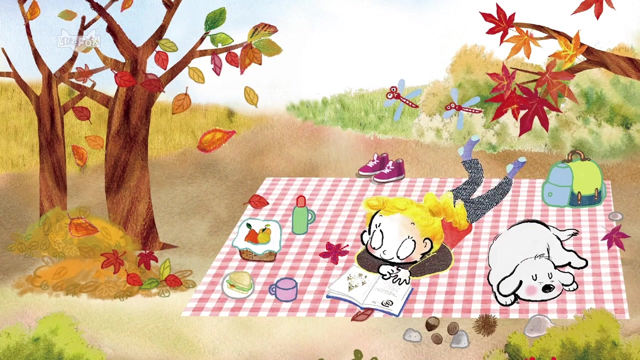 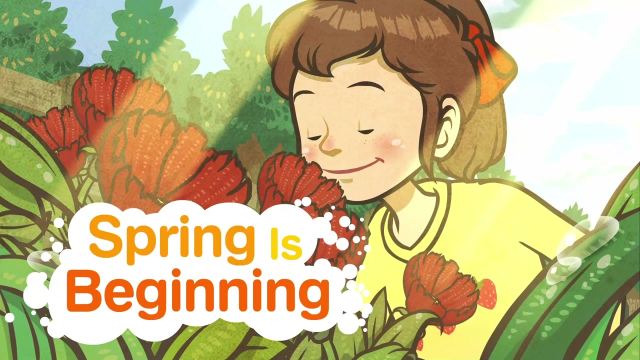 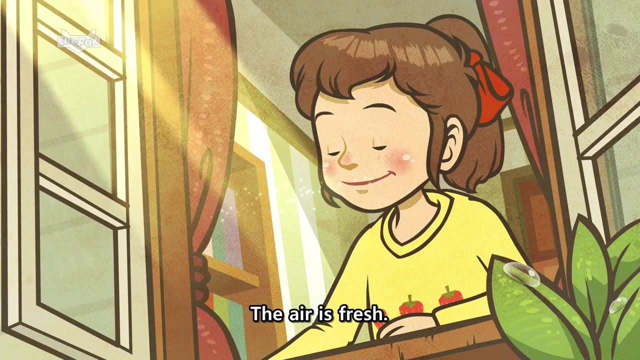 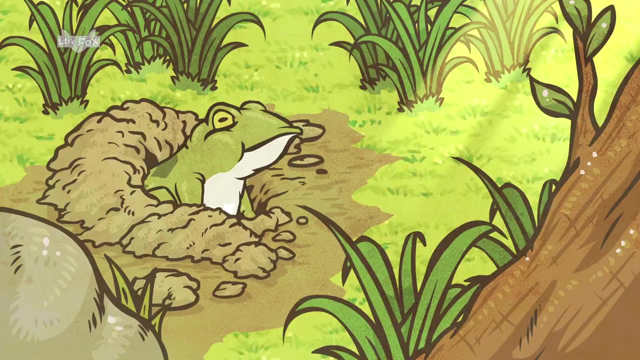 Summertime, summertime, Hot sun, hot sun. Summer is hot. Summer is hot. Now it's fall. Now it's fall, Now it's fall. Falling leaves, falling leaves. Fall is cool. Spring is beginning. spring is beginning. I open the window, the air is fresh, the animals are waking up. I watch the 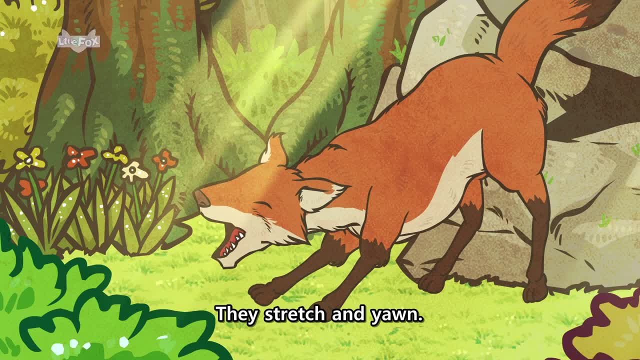 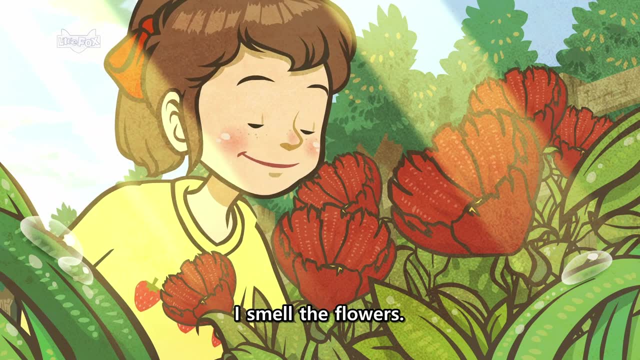 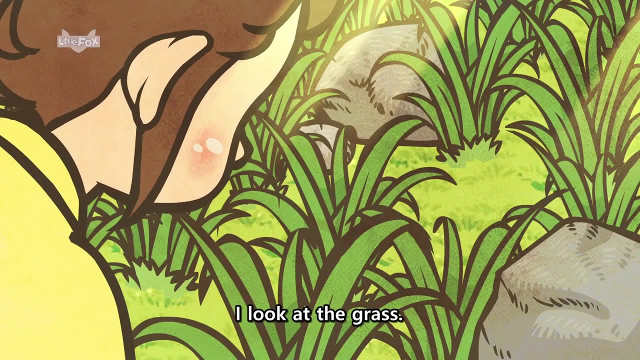 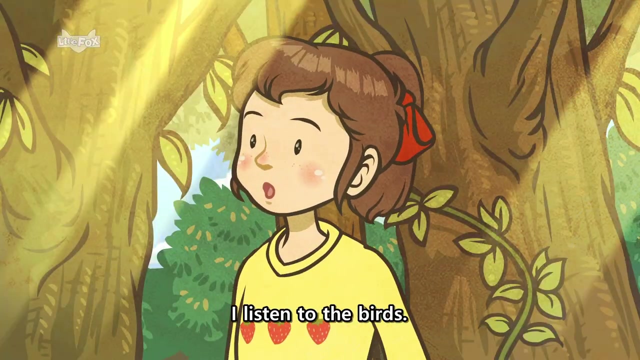 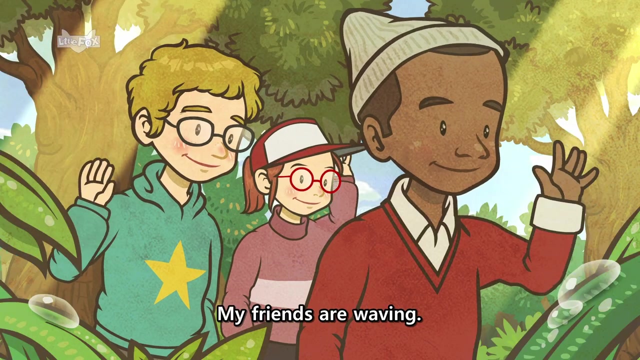 animals. they stretch and yawn. the flowers are blooming. I smell the flowers. they smell good. the grass is growing. I look at the grass. it is so green. the birds are singing. I listen to the birds. they are in their nest. my friends are waving. I wave too. I think about picnics. my friends are. 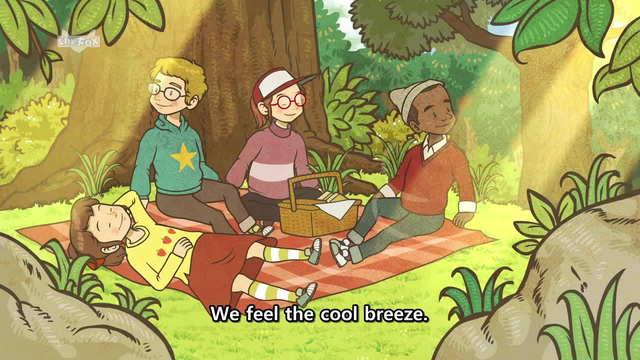 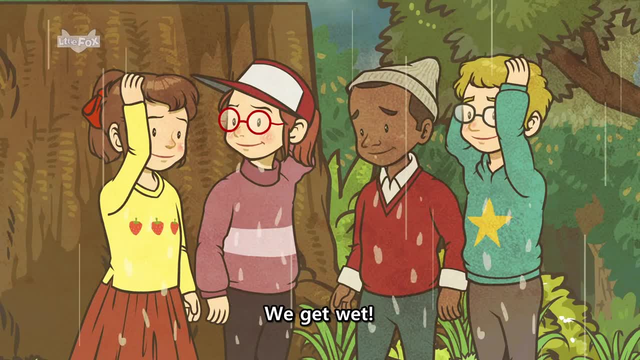 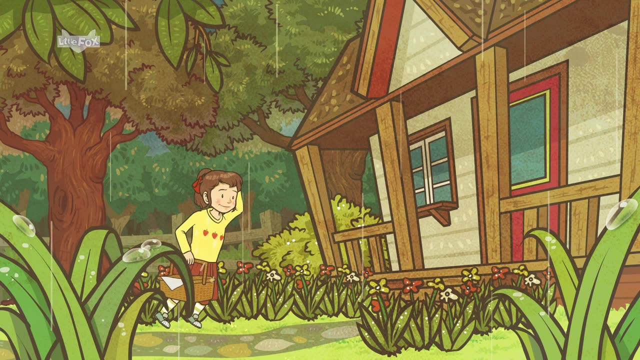 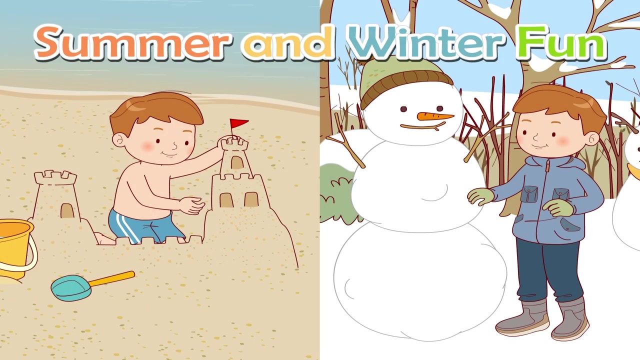 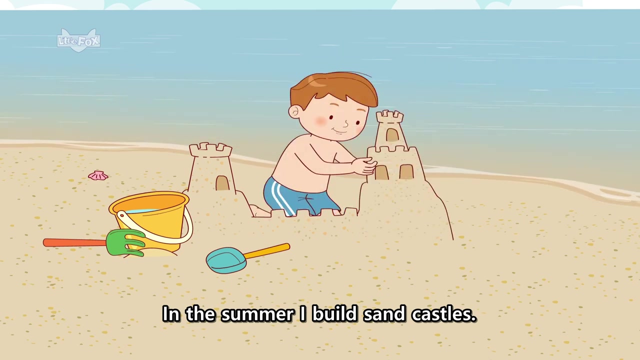 sitting. I lie down. we feel the cool breeze, the birds are singing. I listen to the birds. they are cool breeze. it is raining, we get wet. we say goodbye and run home. summer and winter fun. in the summer I build sand castles. in the winter, I build snowmen. 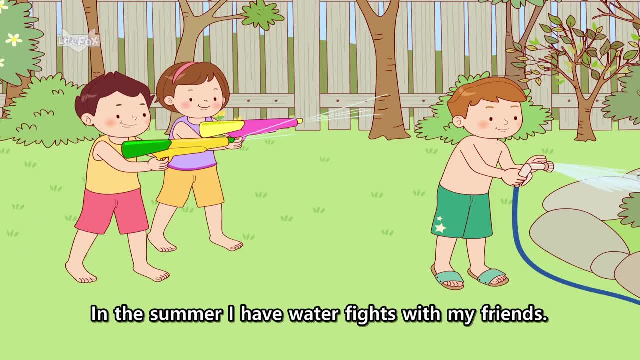 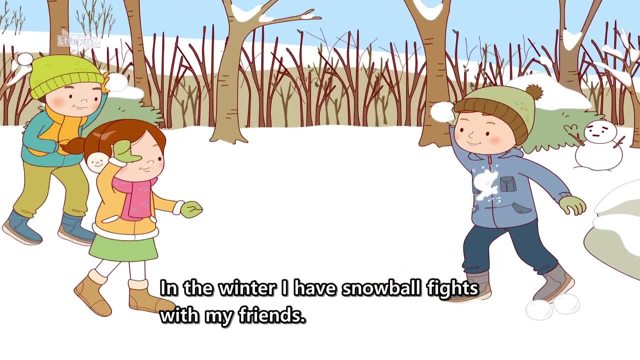 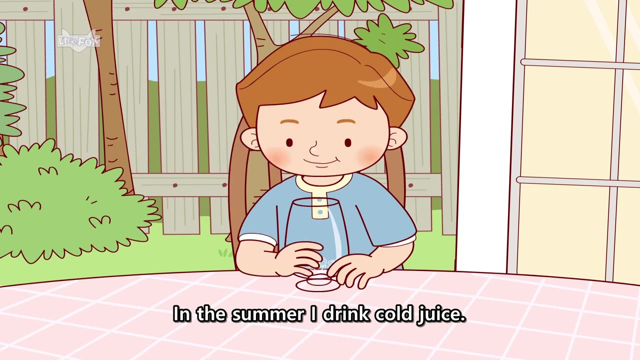 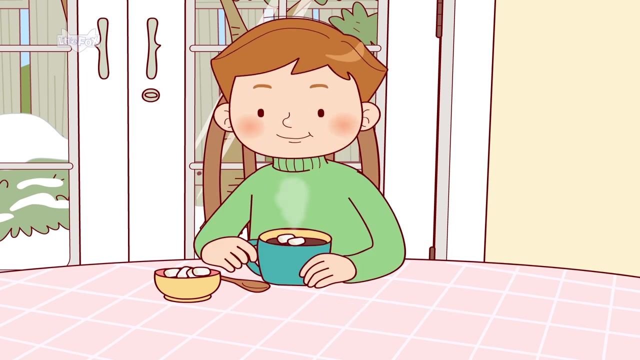 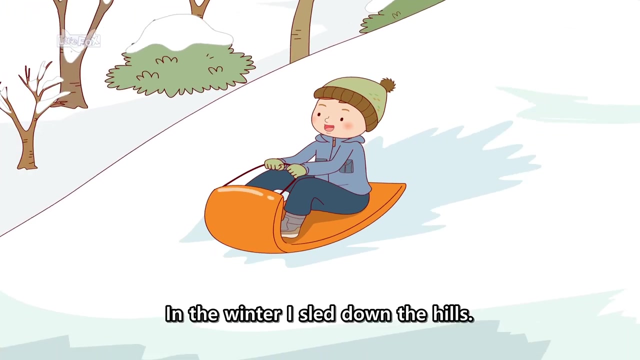 in the summer I have water fights with my friends. in the winter I of snowball fights with my friends. in the summer I drink cold juice. in the winter I drink hot chocolate. in the summer I roll down the hills. In the winter I sled down the hills. 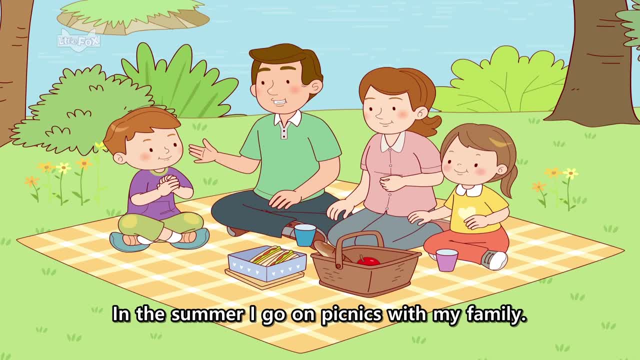 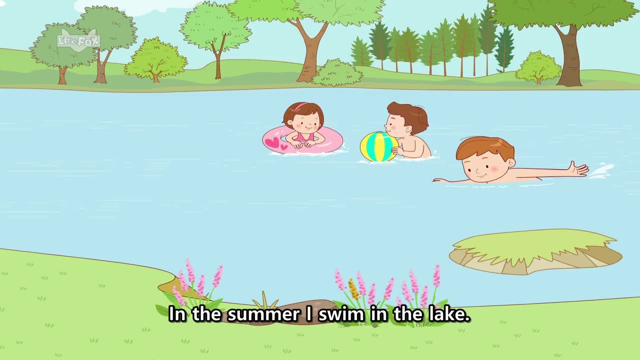 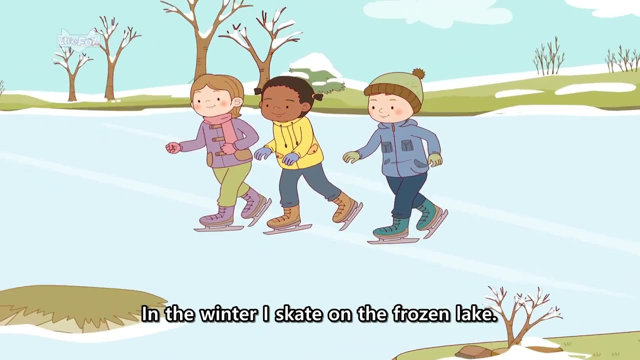 In the summer, I go on picnics with my family. In the winter, I go skiing with my family. In the summer, I swim in the lake. In the winter, I skate on the frozen lake. In the summer, I turn on the fan. 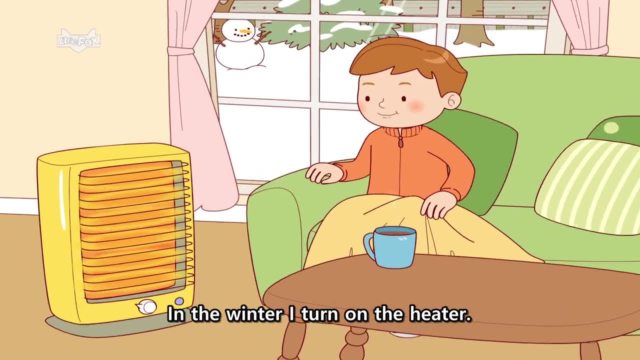 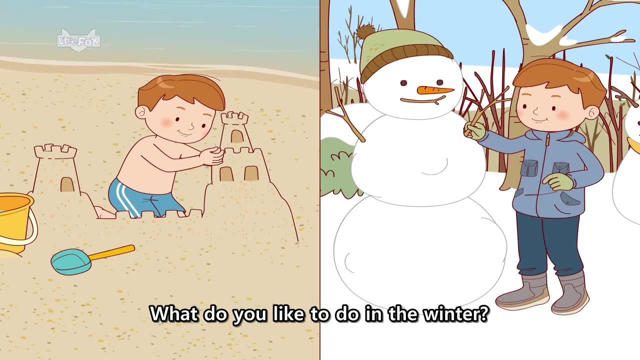 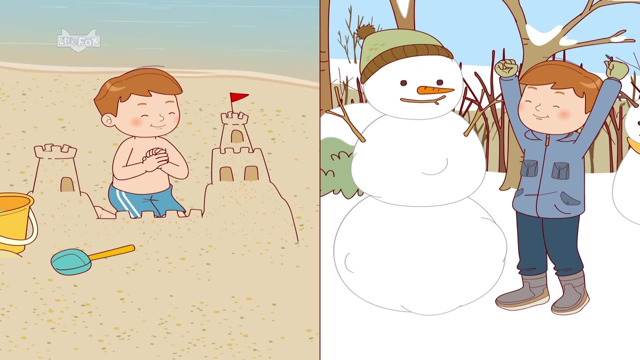 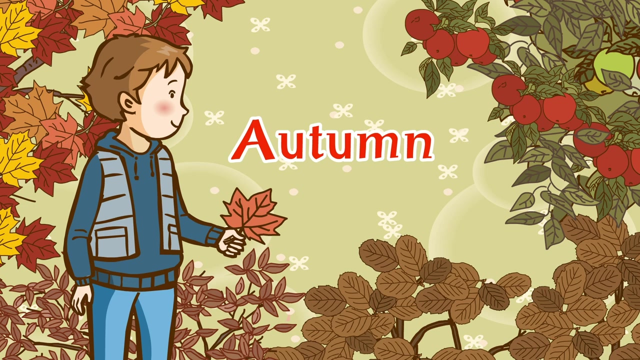 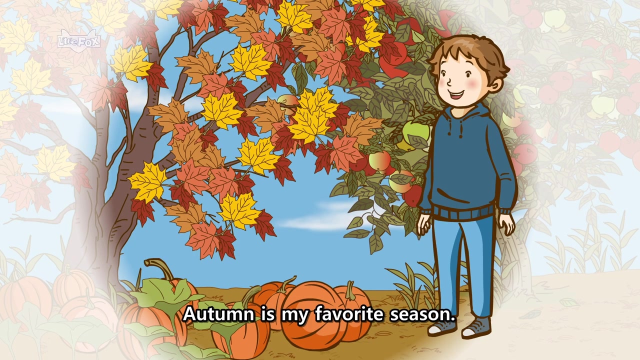 In the winter, I turn on the heater. What do you like to do in the summer? What do you like to do in the winter? What do you like to do in the winter? Autumn is my favorite season. There are so many things to do. 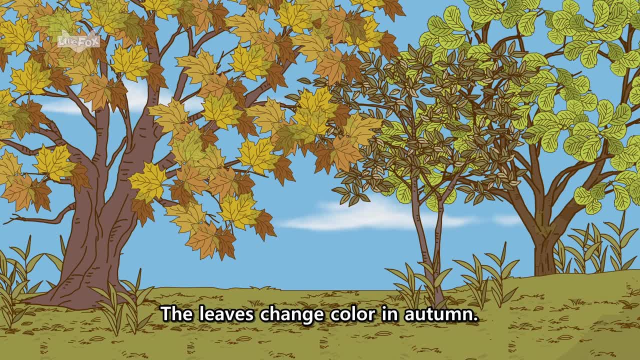 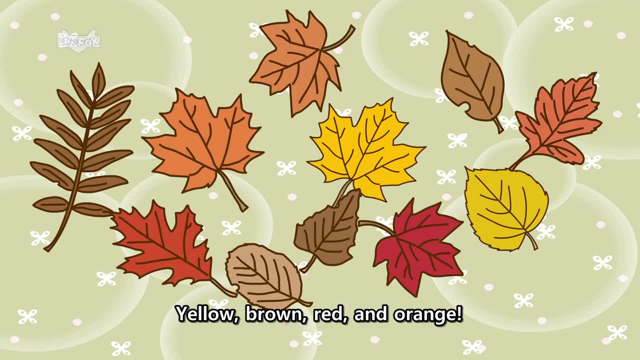 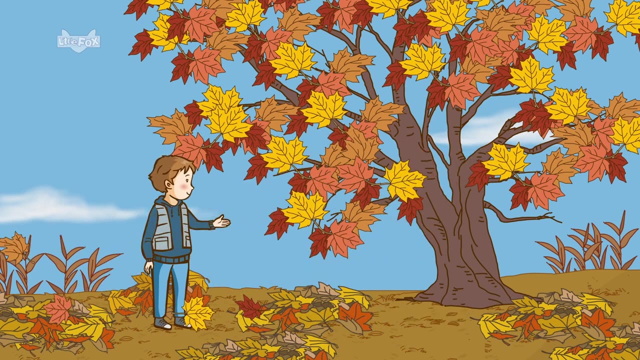 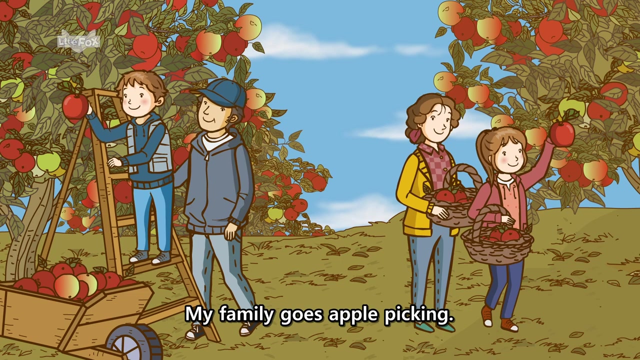 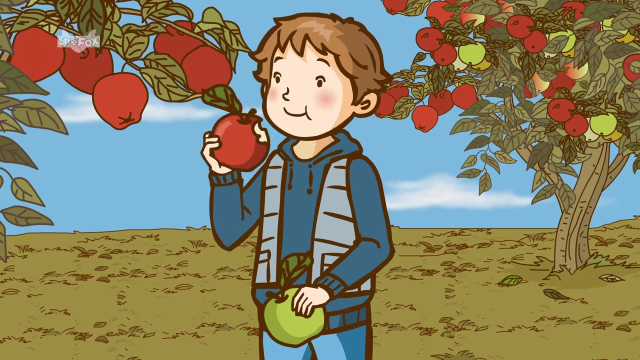 I can't wait. The leaves change color in autumn: Yellow, brown, red and orange. I like to watch the leaves fall down, Then I like to jump in them. My family goes apple picking. This red apple tastes sweet, This green one tastes sour. 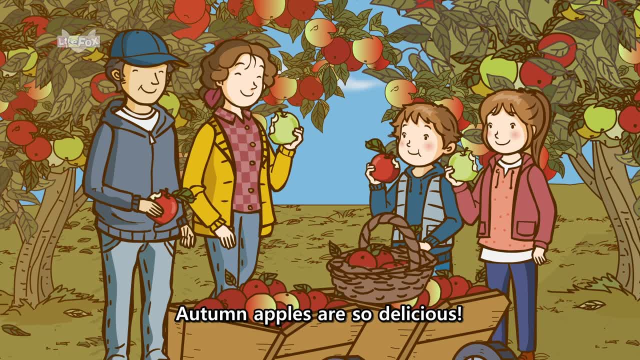 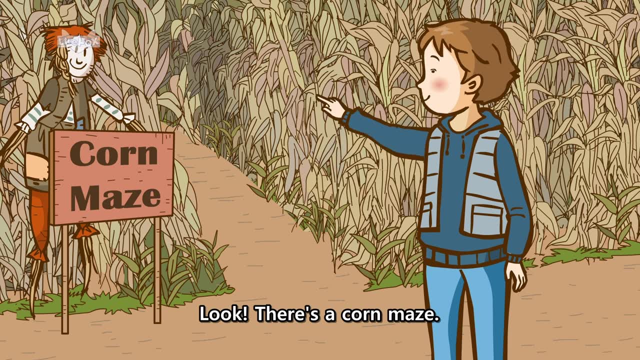 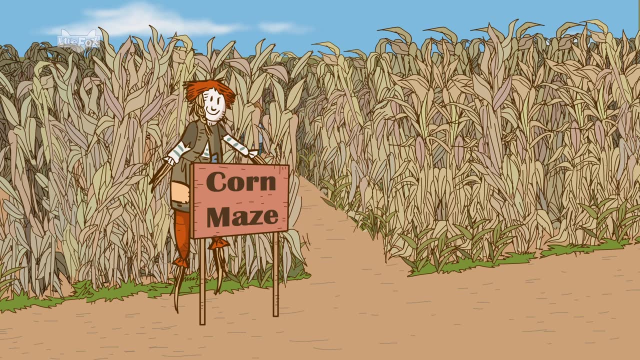 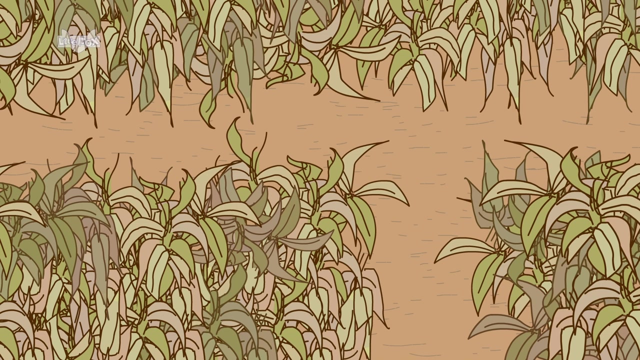 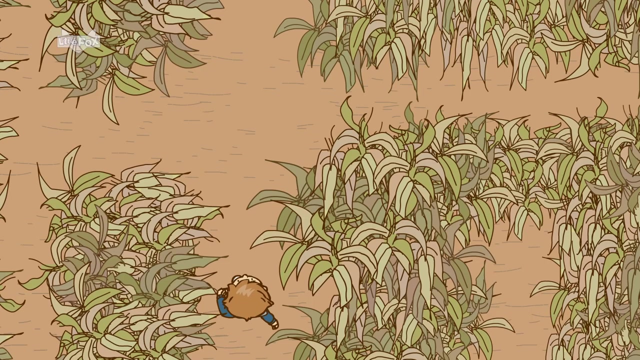 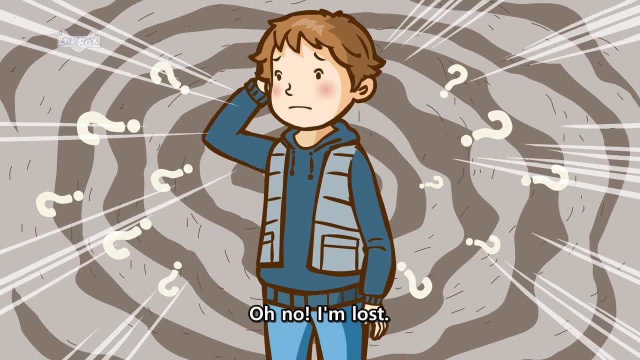 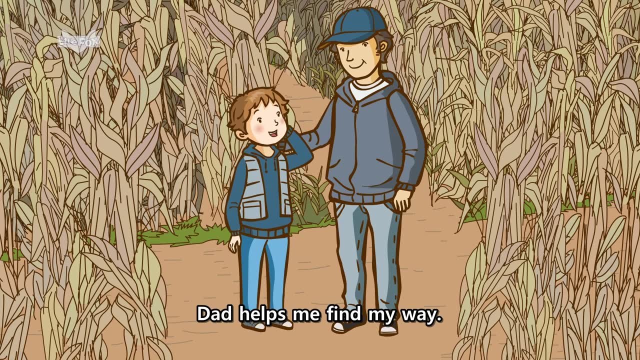 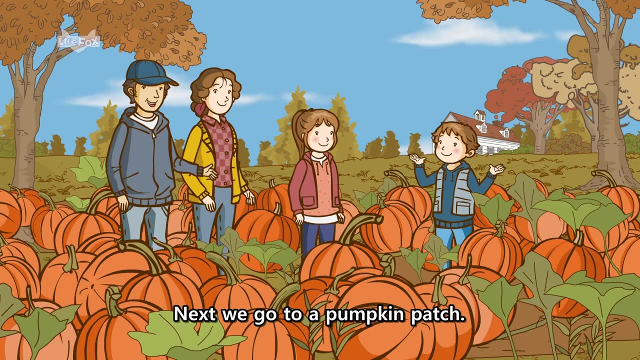 I go right, I go left. Oh no, I'm lost. I only go straight to theủ. Dad helps me find my way. My mother goes with my dad. Next we go to a pumpkin patch. She goes right, I pick the largest pumpkin. 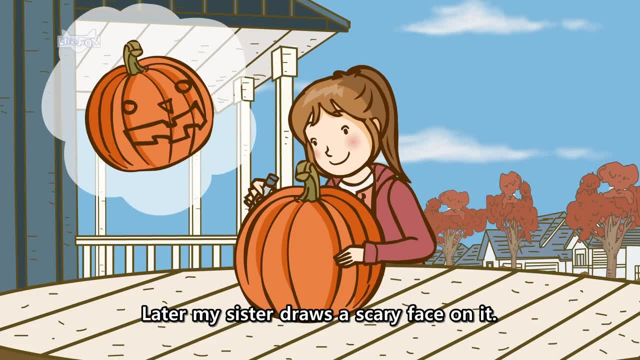 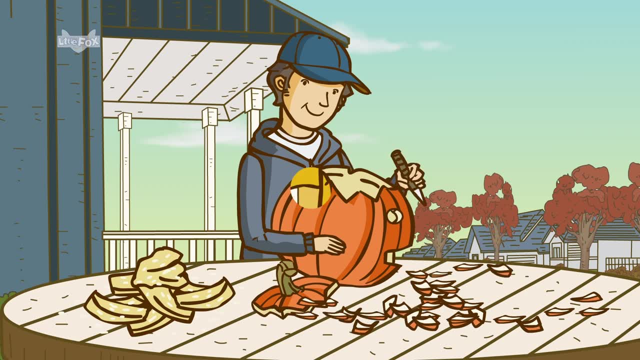 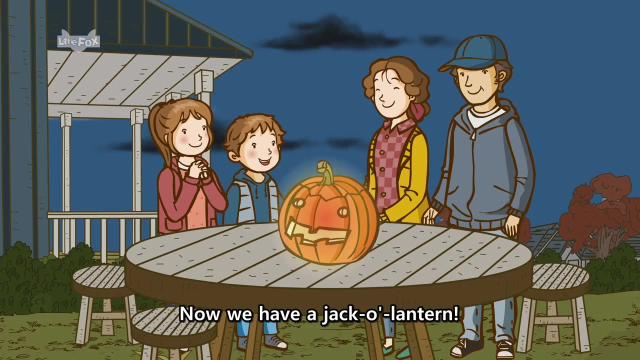 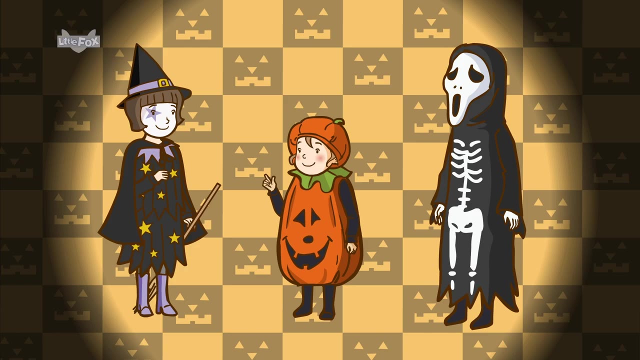 The middle Live hole is a mushroom. Later my sister draws a scary face on it. Dad carves the pumpkin. Mom lights a candle inside. Now we have a jack-o'-lantern. We dress in costumes for Halloween. I'm a scary monster. 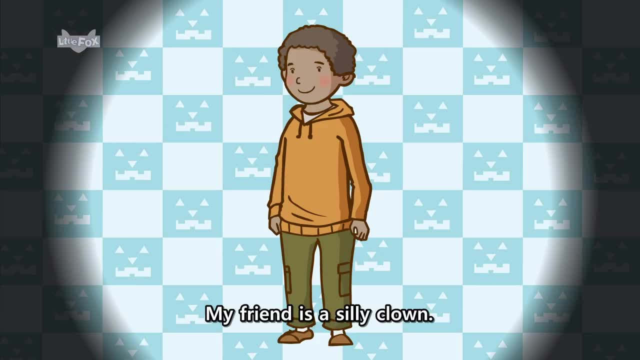 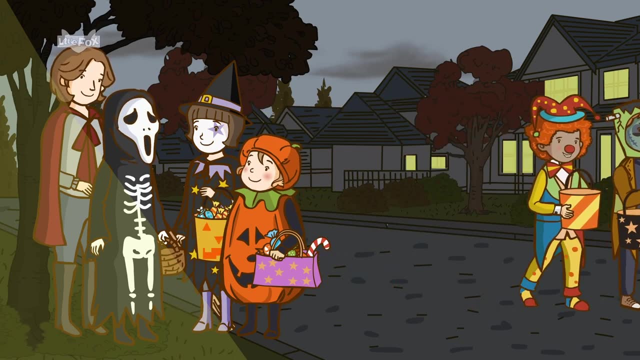 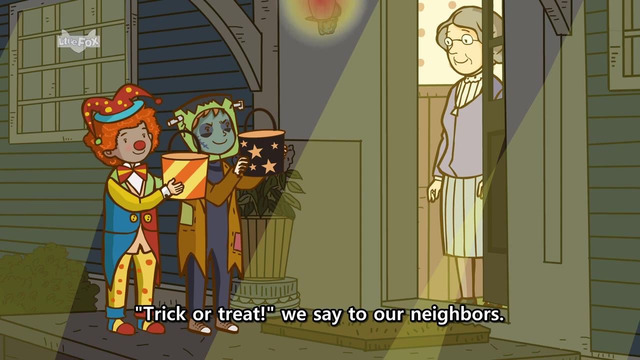 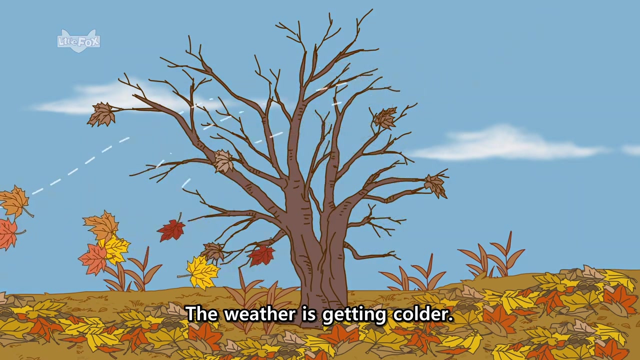 My friend is a silly clown. We walk around the neighborhood Trick-or-treat, we say to our neighbors. Then they give us candy. The weather is getting colder Now. autumn is over. Goodbye autumn. See you next year.